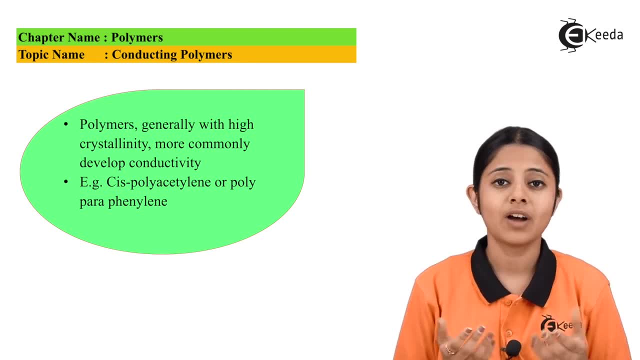 polymers will conduct electricity. Polymers which have high crystallinity in it, That means high crystal formation ability. That means high crystal formation ability, That means high crystal in it- are good conducting polymers or good conductors of electricity. Let us see certain 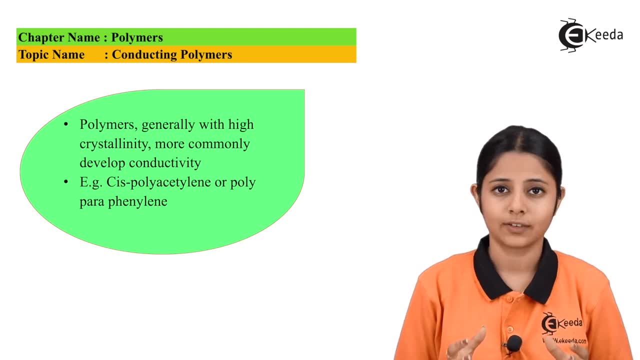 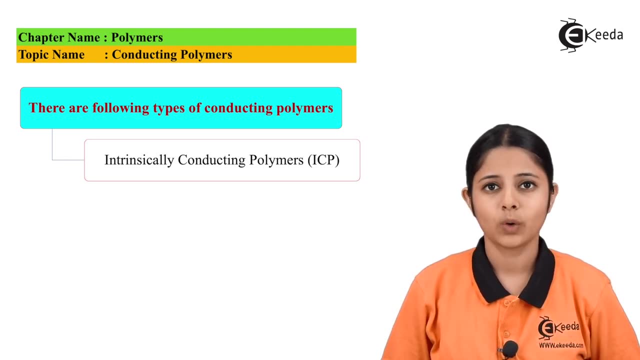 conditions or certain types of polymers which will conduct electricity. The first one is intrinsically conductive polymers. We also call them ICPs. Now what exactly are ICPs? ICPs are those substances which have a pi bond backbone. Now what exactly is a pi bond? Pi bond is a cloud. 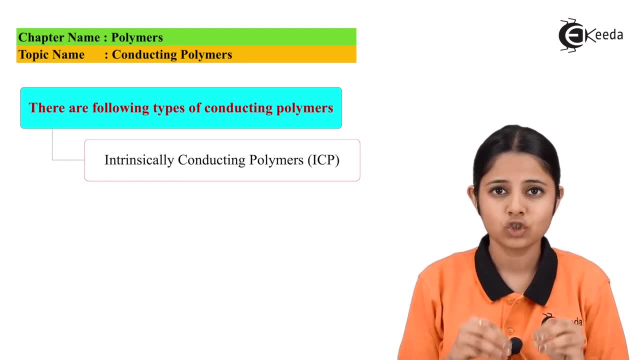 of electrons. There are certain electrons which are extra in a pi bond backbone. So pi bond is a polymer which form a pi bond And because of these excess of electrons these ICPs get the ability to conduct electricity. What is electricity? Flow of electrons from one point to another point. 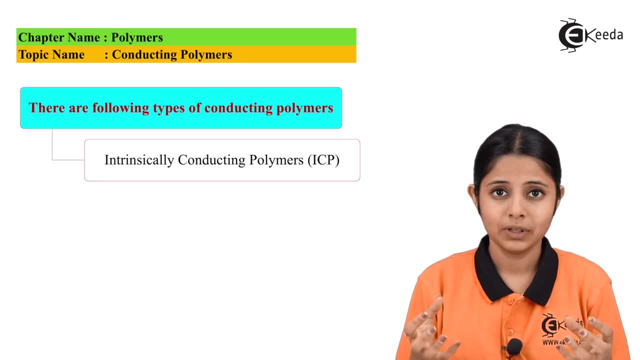 Since these ICP materials have excess of electrons in them, these electrons can flow from one point to another point And because of that flow from one point to another point they conduct electricity. The second type of polymers are DCP, known as doped conducting polymers. Now, what exactly is doping? 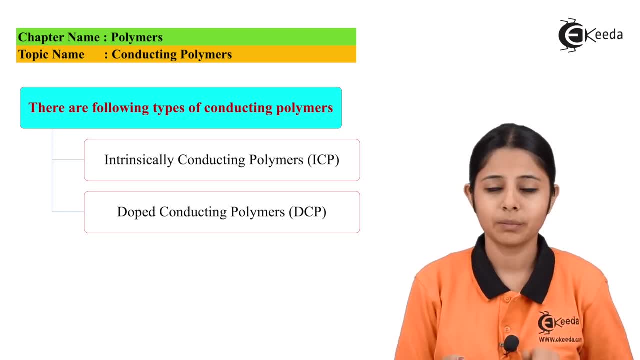 Doping is a process of adding certain impurities inside my material. Now, these impurities can be positive impurities or negative impurities. We should remember that these impurities are added by us. That means those are desirable impurities. Because of the addition of those impurities, 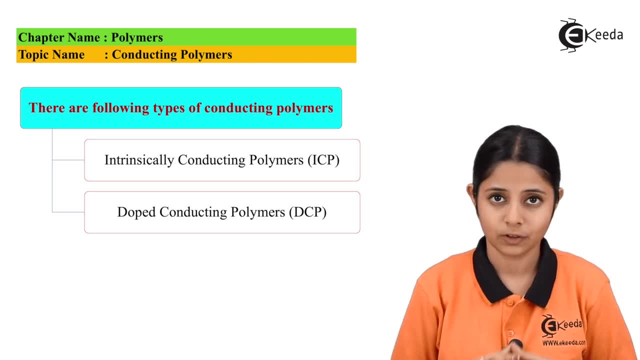 that particular plastic or a particular polymer will start conducting electricity. Now, to start conduct electricity, we provide certain ions to it, Positive ions or negative ions. Positive ions are known as anions. If positive ions are present in it or cations are present in it, we call it as. 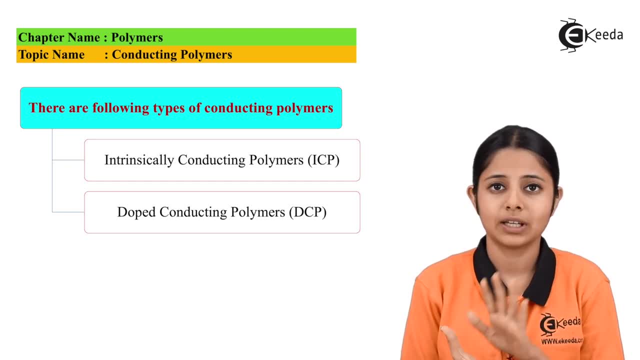 p-doping, That means positive doping. Some positive impurity has been added. If negative ions are present in it or anions are present in it, we call it as n-doping, which is negative doping taking place for that particular plastic or polymer. So the next one or the third one is extrinsically 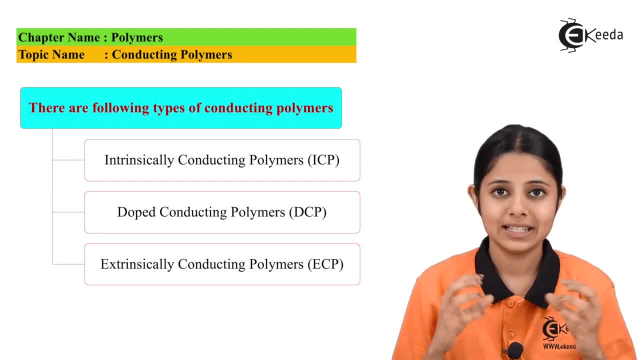 conducting polymers, also known as ECP. Now these ECPs are of two types: One is called anion and two types: CEFP and BCPs. CEFPs are conducting element filled polymers and BCPs are blended conducting polymers. Now, what are these polymers? Conducting element filled polymers? CEFPs means.